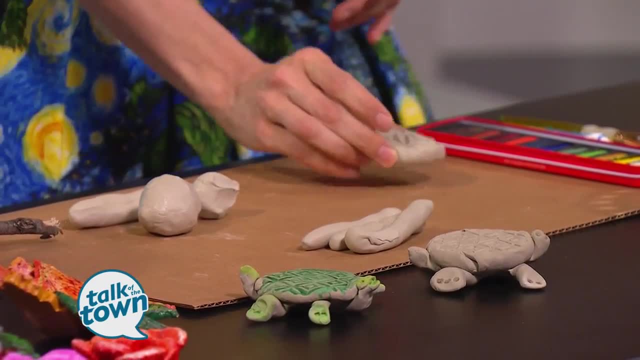 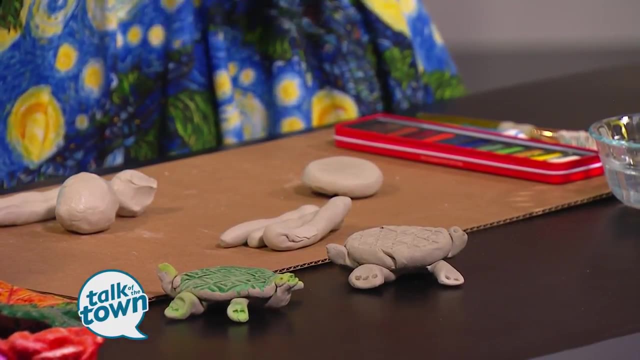 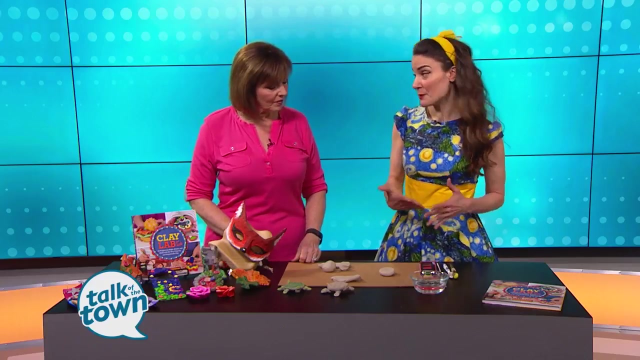 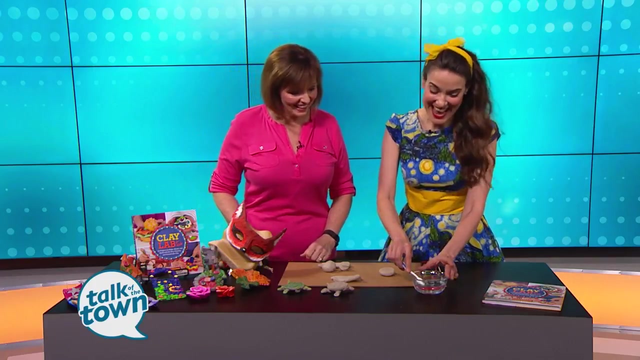 then that makes the turtle shell. Yeah, that's the turtle shell. You flip the turtle shell over and when a traditional clay artist is working with clay, they do something called slip and scoring, which means they scratch into the clay. add a little bit of water or watery clay and that's how they attach. That's the glue that holds it together. That's complicated for kids, Sure. So one method in the book is for them to use an old toothbrush- preferably not mom or dad's Right- And just to get that wet, and this scratches into the clay while creating something called slip, which is that 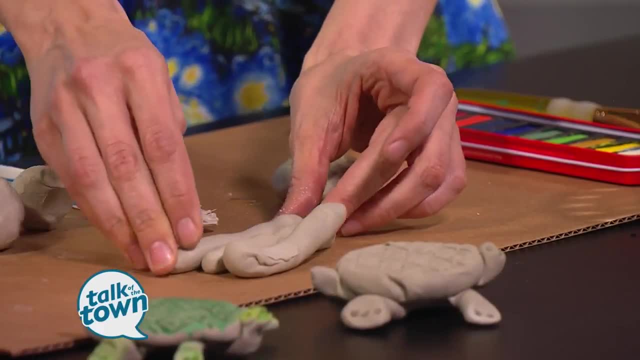 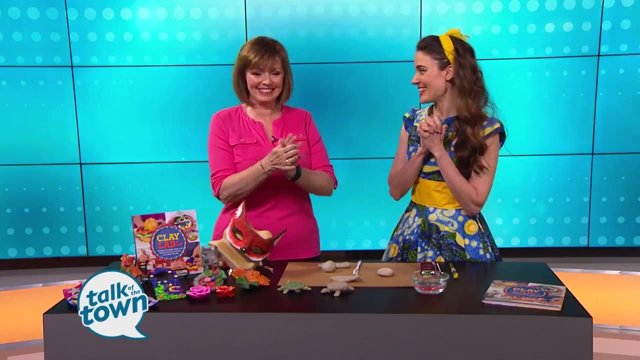 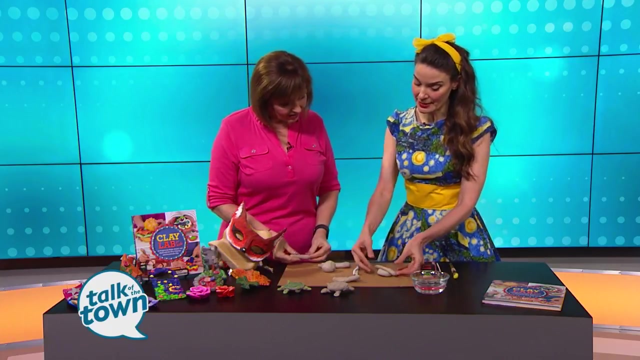 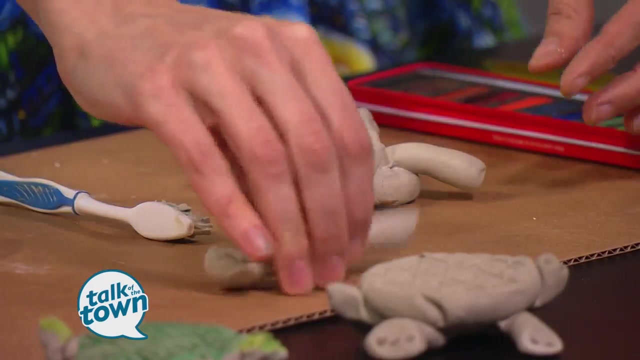 watery clay And then, once that's done, that acts as the glue. Then they're to take clay and roll something called coils. So that's, when you just roll it up, It's a clay snake. Yeah, Essentially Yes, Getting all nice and messy, And then, after they have three of those, those are then just kind of placed like a diagonal line, smoosh it into the clay, then create an X for another one, And then the last one goes right across this way: Oh, and that's head and tail. You got it. So then, when they flip it over, they've got. 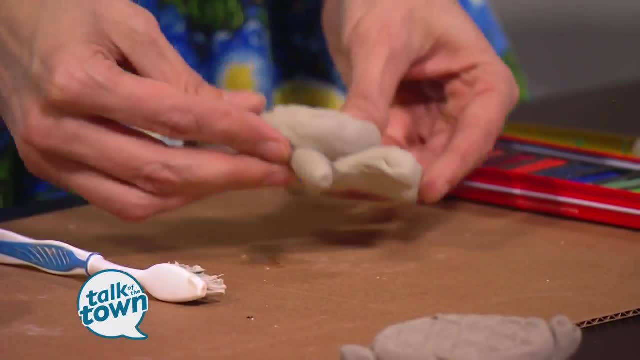 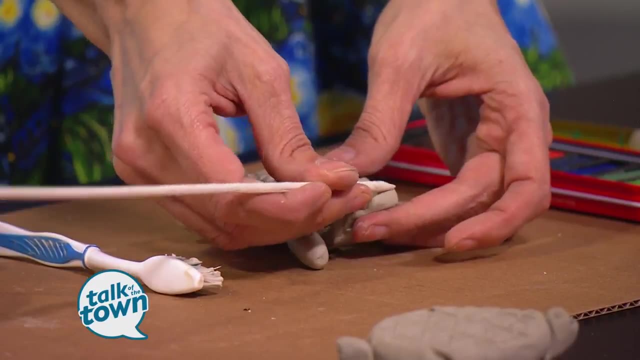 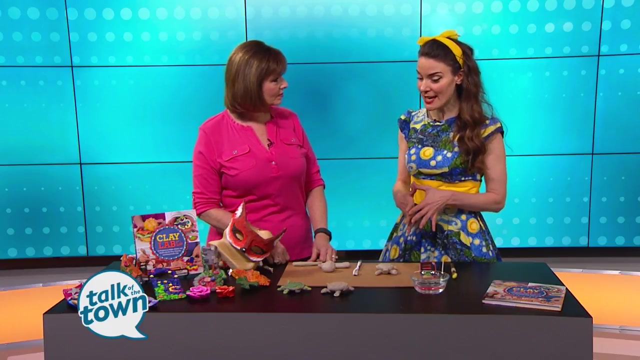 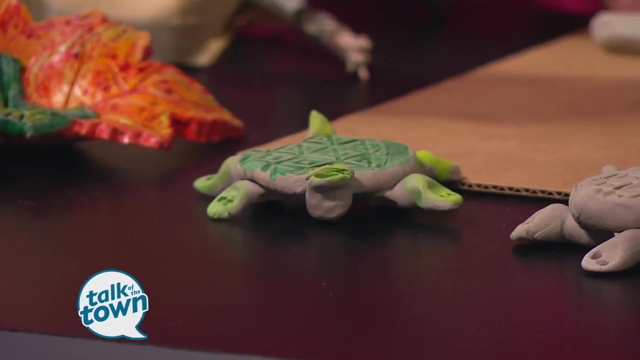 the start of a turtle, So it looks a little bit like that, Yeah, And then we use a lot of skewer sticks that we can create designs like the eyes and then maybe go horizontally And then you've got a mouth. Oh, that's a really fun, simple, quick project And it's great for kids to see that clay is something that captures texture, which is one of the coolest things about it. That's great. So this is a project that would work for four or five year olds probably. Oh, yeah, I did Like I said, my kindergarten kids, But then the fascination of just stepping on the clay- my second graders did as well. 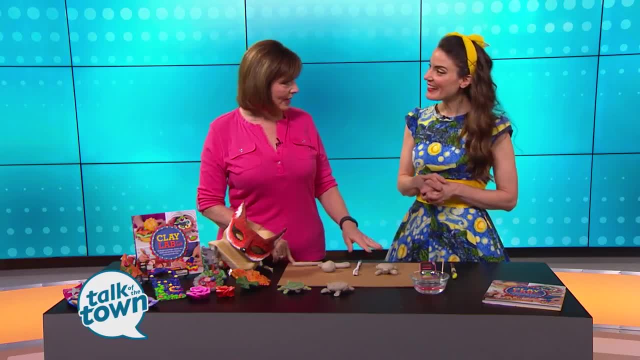 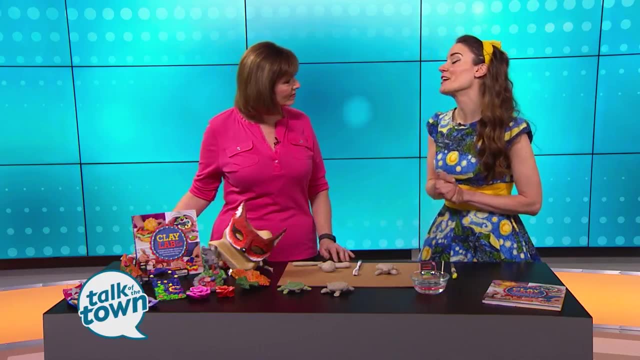 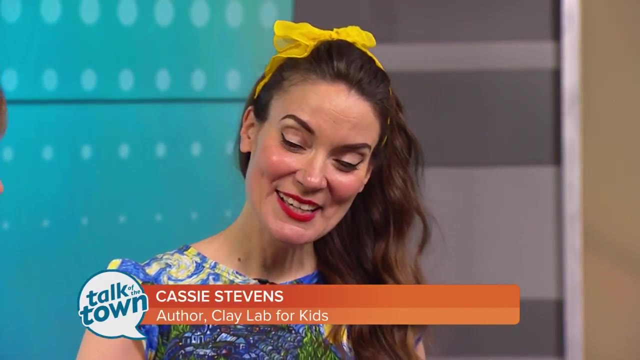 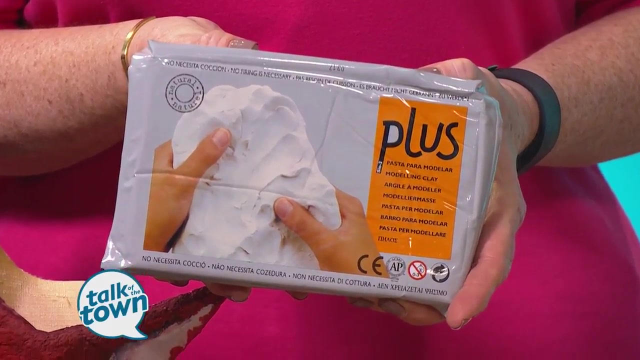 And they had a great time. That's cool. Yeah, All right. So this doesn't need to be baked or it just air dries, Correct? This is an air dry. clay usually takes a couple of days, especially, you know, humidity in Tennessee. You might want to put a fan on it because it might take a little bit longer. And I want to show you this clay too, just so you know when you're looking in the craft store for it. It's plus clay, It's made by Activa And it's a great clay. But you know what? There are so many different kinds of air dry clays at the craft stores that really I've used just about all of them in the book.